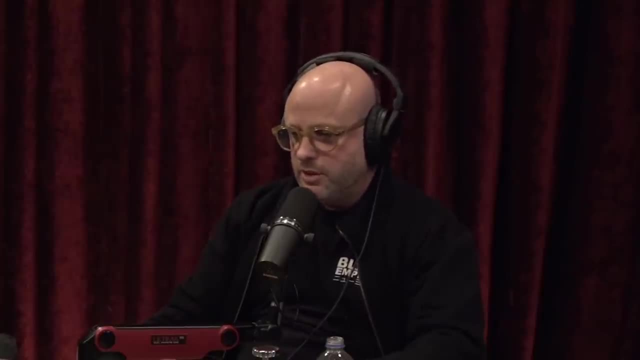 And he came down. He's got a couple of restaurants up in San Francisco Bay Area. He's he's an amazing chef, He's a great travel buddy And I was just yesterday. I was like, I mean what, Talk to me about culinary school. 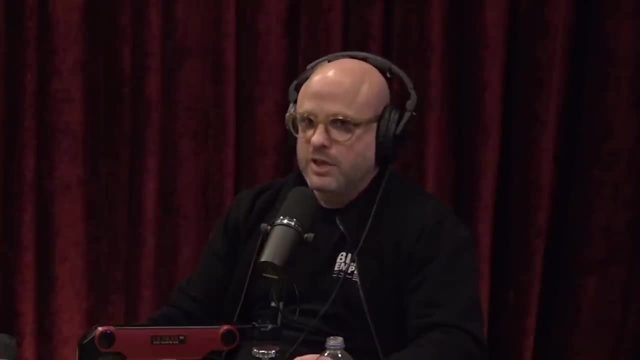 Like, what do you think? What's our opinion about that? Like, because I went to culinary school. I dropped out. I didn't make it through. He went to culinary school. If you want to be a chef, I don't think culinary school is necessarily the best route. 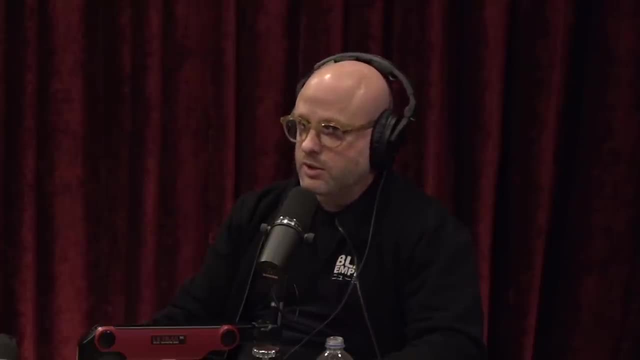 If you want to be a chef of an independent restaurant, If you want to work as a, If you want to be a home cook. there's a lot to learn quickly from culinary school. I think that's good as a, as a non matriculated kind of class by class. 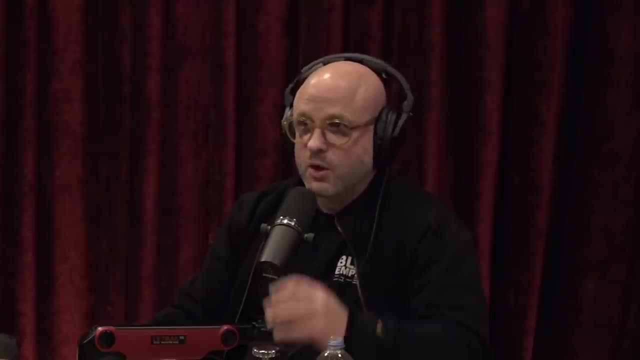 There's a great, that's a great opportunity Taking some cooking classes as a home cook. You learn a lot If you want to be a chef. it's a hands on experience in the restaurant that's going to get you there. But I think there's a lot there's, if I think there's definitely a use for taking cooking classes as a home cook. 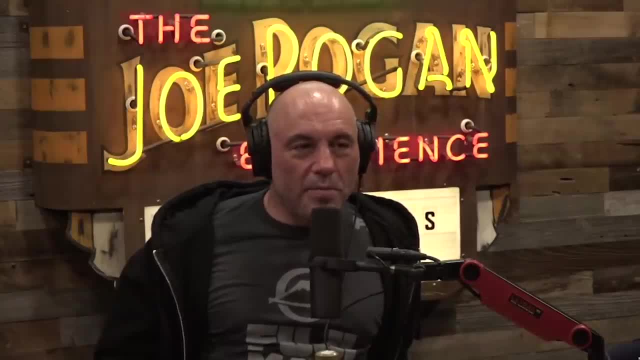 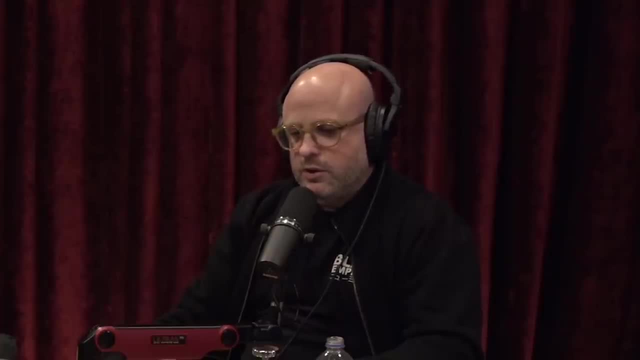 You're not the only one who's told me this. This is that that sentiment has been echoed by a lot of great chefs that have Talked to said the same thing. My problem is also, though you know for a certain, there are a lot of culinary jobs out there. 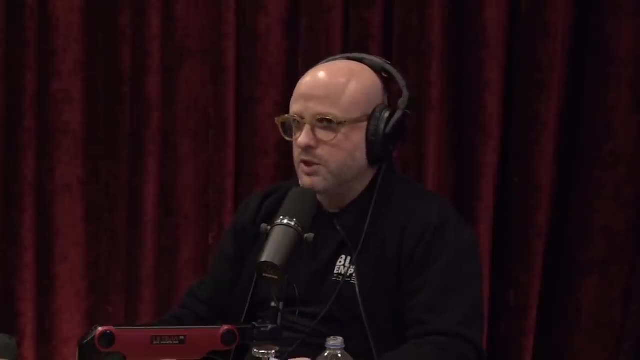 And you know, think about all the hotels and all the cruise ships and all the corporate cafeterias. There's so many culinary jobs out there And if that's a goal, if you want to work in one of those jobs, then culinary school can be a great road to give you the, the, the needed. you know that can be a great route to get one of those jobs. 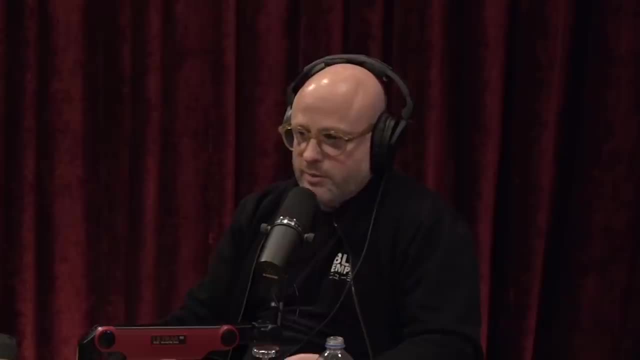 If you want to have a stand Alone restaurant, maybe something more avant garde, maybe something where you're, where you're a little more creative than culinary school, might not get you there And it can put you at a disadvantage because you get, you know, unless you like, I got, I was very lucky. 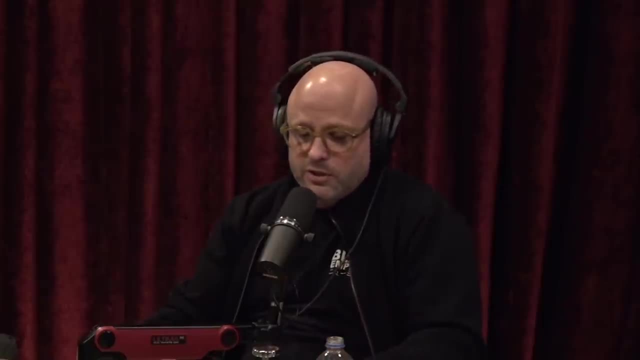 I got a full scholarship. The James Beard Foundation gave me a full scholarship to go to culinary school, And so it worked out for me. But for so many folks like you go to culinary school, you come out with big debt and then you can't afford to take a job at a restaurant that's paying minimum wage. 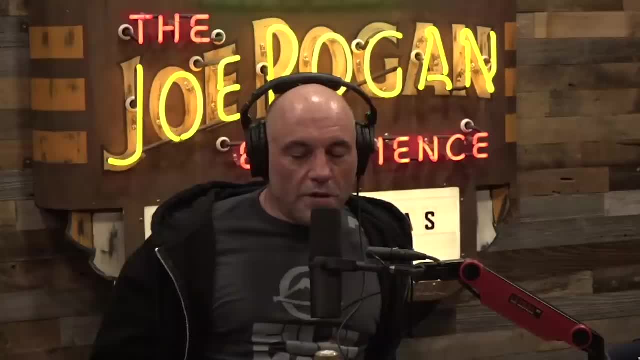 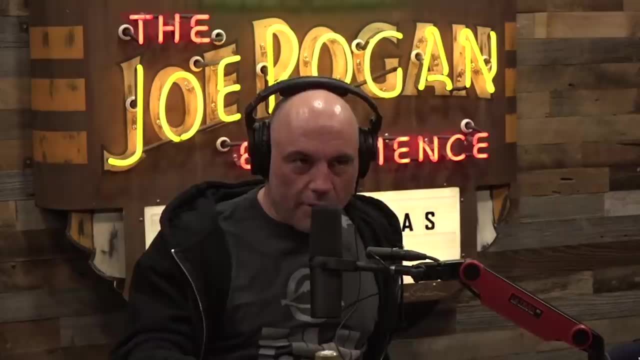 Because you need to pay back that loan. So if you get a job at a restaurant, the restaurant will essentially give you a task And then if you show effort and show that you have work ethic and show that you're really interested, they'll slowly train you to learn new techniques and cook things. 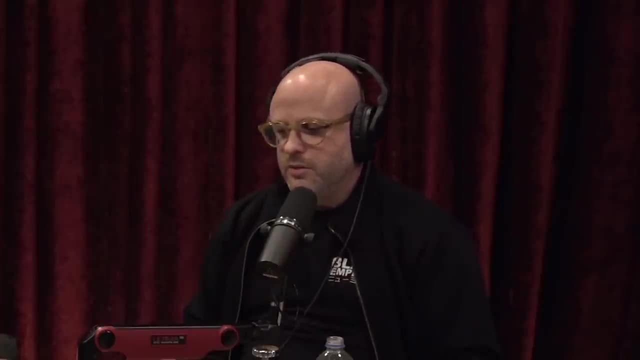 I guess- And this is this- gets into like a whole nother issue that's going on right now with the labor laws and how they've really kind of changed the way That people in restaurants learn how to cook and cooks come up in the business. 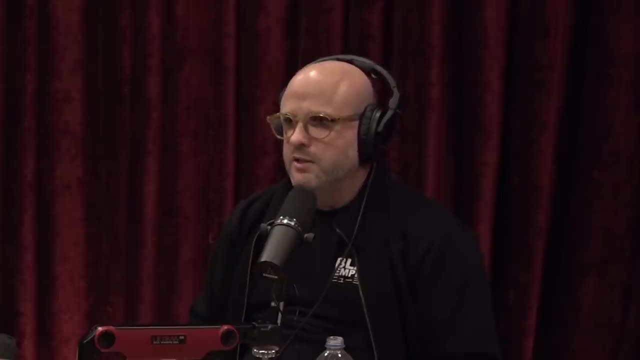 So I kind of came up at the end as the last of the end of the world where the apprentice system was still kind of a piece of the puzzle, if that makes sense. So I went and worked at Le Bernardin, super fancy French restaurant. I was, like, you know, 15 years old, 14 years old, And I, you know, I, chef, was like I can't pay you. You know you're not legal to work, but you can come and work for free. So did you always know that You wanted to be a chef? I love to cook, And when did you start? I started when I was very young. I have pictures of cooking with my mom, Very, very young, And she, she kind of supported me in that. 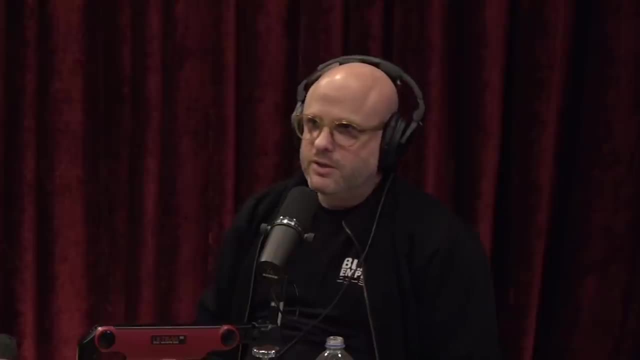 So we had, you know, making pasta in the kitchen and hanging the noodles off the back of chairs and having you know she was very, very supportive of of my interest. When I was 13 years old, I got a job delivering pizza at the pizza. 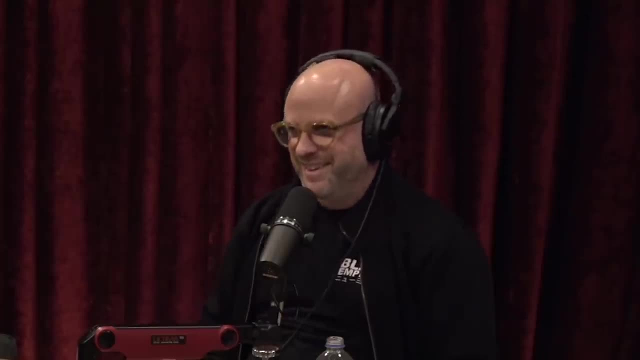 Pizzeria across the street: Gino's Pizza. Vincent, How did you deliver them on a bike? I was walking and I had a harmonica. I would play the harmonica. I thought I was the coolest kid in the world. 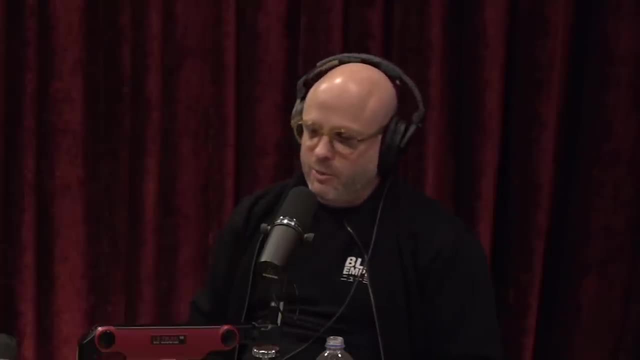 It was not cool. Meanwhile, my partner, Michael, who I ended up opening a restaurant with Michael Michael's- you know who. we should talk about him to you. This guy's, he's very cool guy, Very inspirational He was. he was a cool kid. 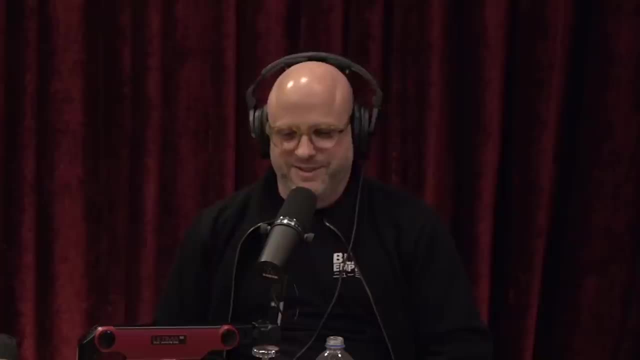 He was delivering on rollerblades, making twice the tips, quick, getting around, you know, But delivering pizzas. And then I was working at this Mexican restaurant, Sam Alita's. I was delivering Mexican food and I was like man, these guys in the kitchen are so cool. 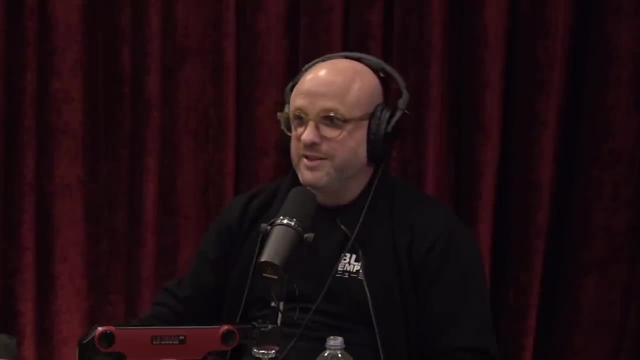 Like got tattoos and the fire and like everybody says yes, chef, And you know, I just I was really attracted to the kitchen and I started. I started spending time in the kitchen and I was working at this vegan restaurant. Mike Mike was delivering. 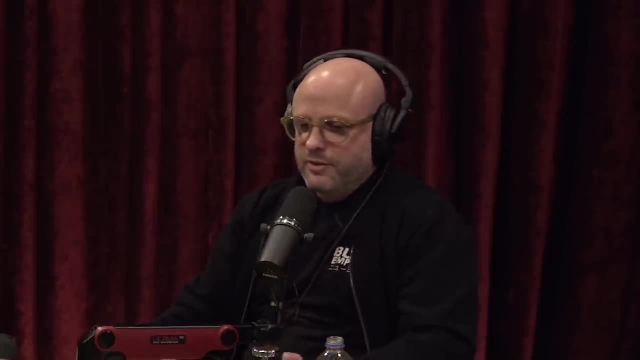 He was, so he was delivering vegan food and other things, So on his rollerblades was like 14 years old. Yeah, it was like a green machine selling weed. He was like son of a bitch. You just order your like your, your vegan vegan seven layer dip, and you get a bag of bag of at the time 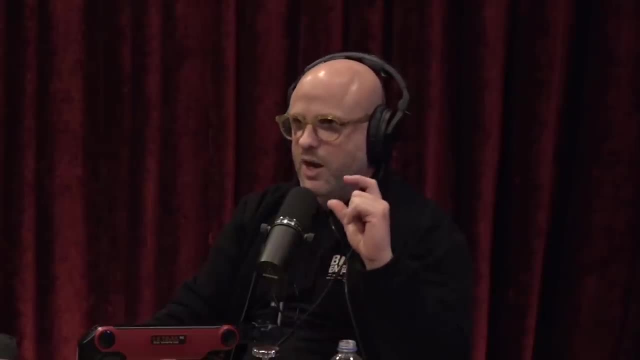 It was like I don't know. it was like the first time that they had a chronic. They called it chronic, like fresh and green, And this, this. I was in love with this, this girl She was, she was amazing. My best friend at the time. 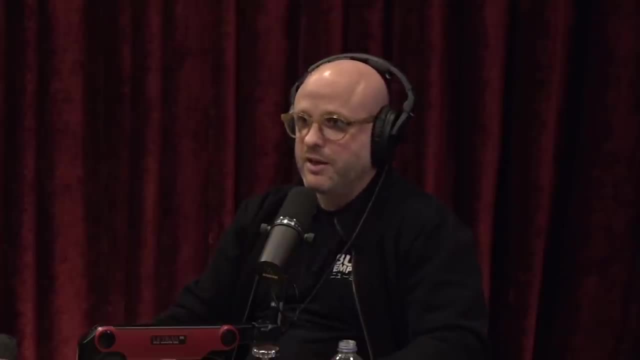 And her father was the maitre d This fancy friend French restaurant. He came in and I was working in the kitchen, because whenever I wasn't delivering I was in the kitchen. I loved it. You know, I was like learning everything I could. 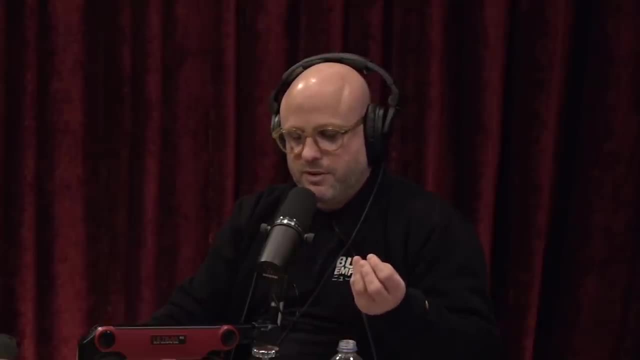 And the chef had just cut herself, you know, like just cut herself and she had to leave. And they were like we got to close the restaurant And and I was like oh, there's like two more dishes to go out. 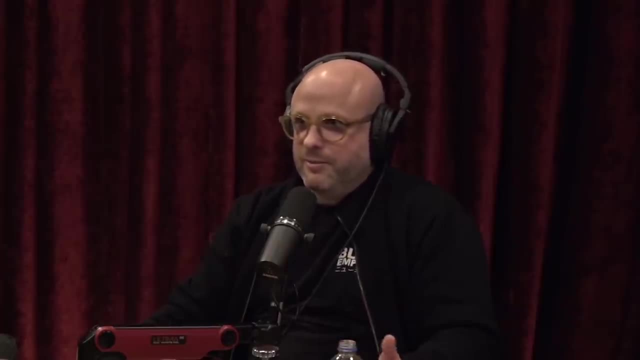 And he came in. He was like I was the only guy in the kitchen. It's like busy restaurants full. He's like 14 year old kid friend of his daughter's. He's like you know, you're the chef here. 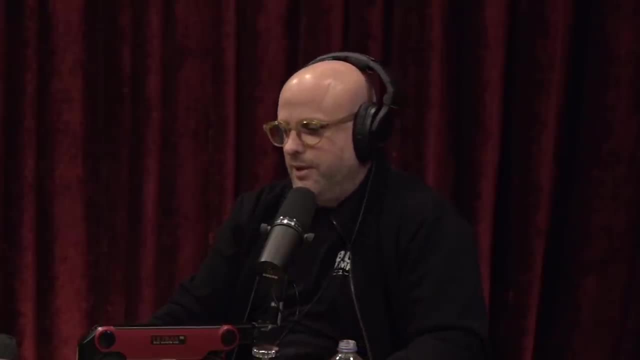 And I'm like, yeah, Like absolutely, He's like you should come I work at this fancy French restaurant. You should meet the chef. And he got me an interview and I went and worked there. So, like 15,, 14 years old, I go and work, go to this fancy French restaurant. 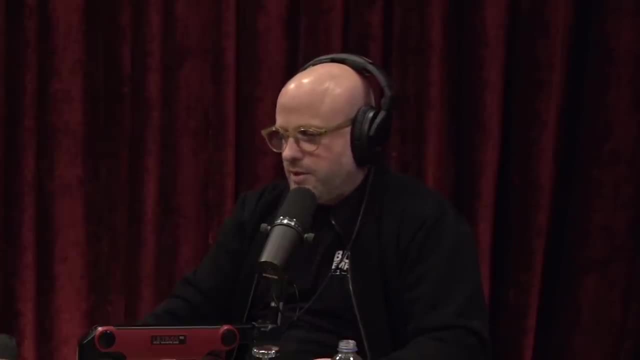 I had no idea. after school and the chef meets me and he's like he's late. He's like you're lucky because I was taking a haircut, because otherwise you would be fired already. I was like, oh my God, I have no idea what's going on. 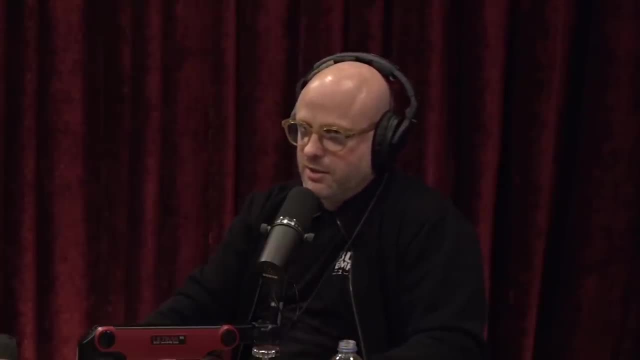 And he's like: but you can come and you can watch Like you, I can't touch anything, You can watch after school. on Wednesdays You come and on weekends. I started working there and it was fun, man, It was super cool. 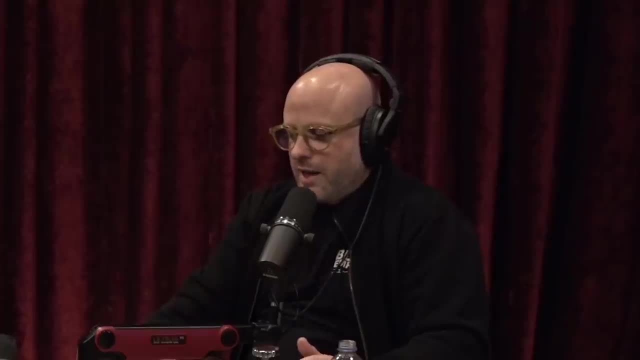 What kind of tasks did they have you do? initially, The first job was I got to bring the fish from the refrigerator to the guy that was going to cook the fish, Like I could carry it across the kitchen. and then I got to clean calamari. 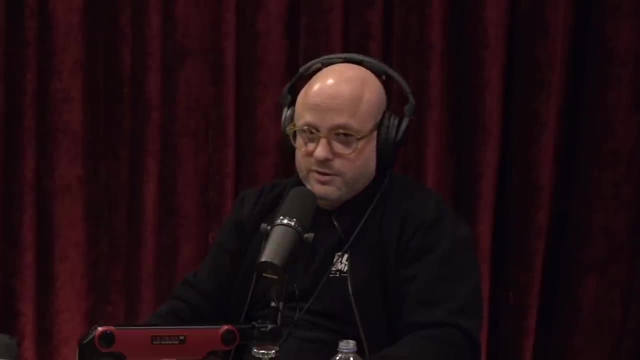 My dad called me the calamari kid. He was like he had a whole, whole, whole song for me. I was like the the squid kid. Um, I remember one time I went in and I was like the chef was like you know, the calamari. some of it has gone bad.